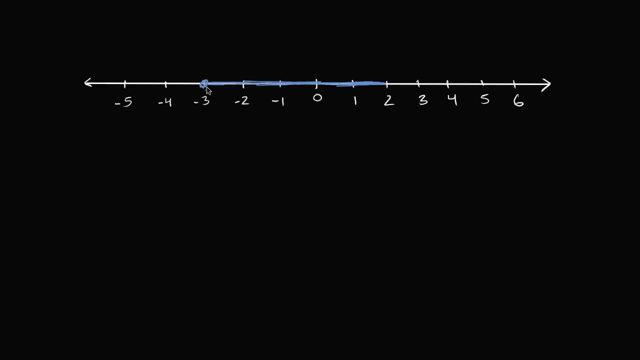 negative three and two, then I would fill them in. So this right over here I'm filling negative three and two, in which means that negative three and two are part of this interval And when you include the endpoints, this is called a closed interval. 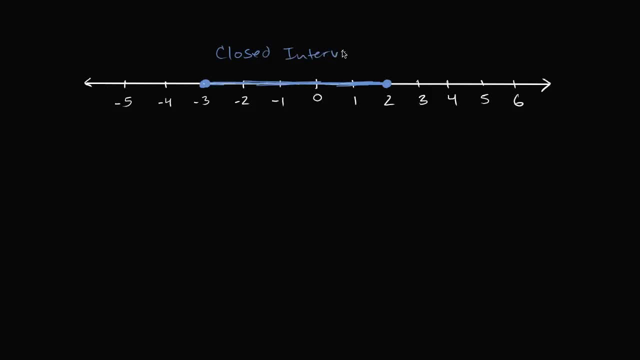 Closed interval. Closed interval, And I just showed you how I can depict it on a number line by actually filling in, filling in the endpoints, And there's multiple ways to talk about this interval mathematically. I could say that this is all of the 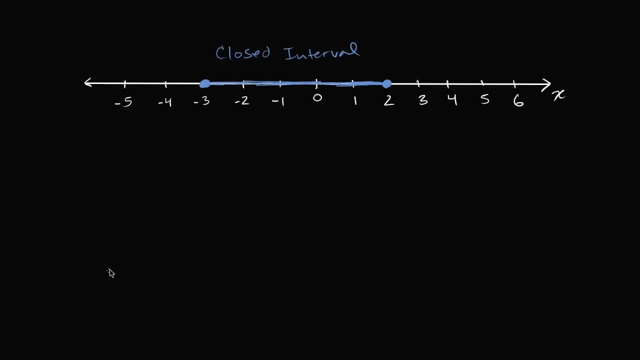 let's say that this is, let's say this number line is showing different values for x. I could say these are all of the x's that are between negative three, negative three and two And two- And notice I have negative three is less than or equal to x. 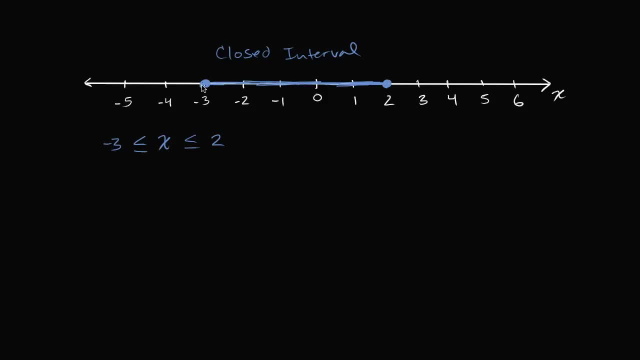 So that's telling us that x could be equal to that. x could be equal to negative three. And then we have: x is less than or equal to positive two. So that means that x could be equal to positive two. So it is a closed interval. 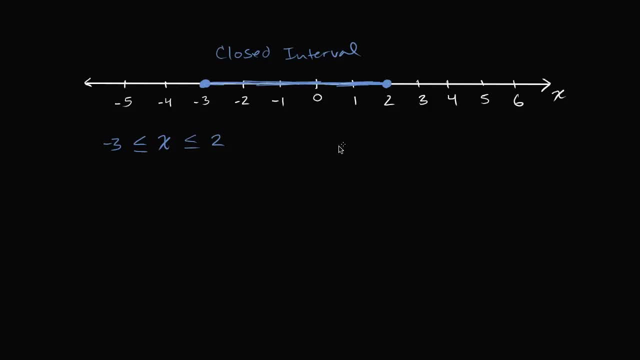 Now, another way that we could depict this closed interval is we could say: okay, we're talking about the interval between, and we could use brackets because it's a closed interval- negative three and two, And once again I'm using brackets here. These brackets tell us: 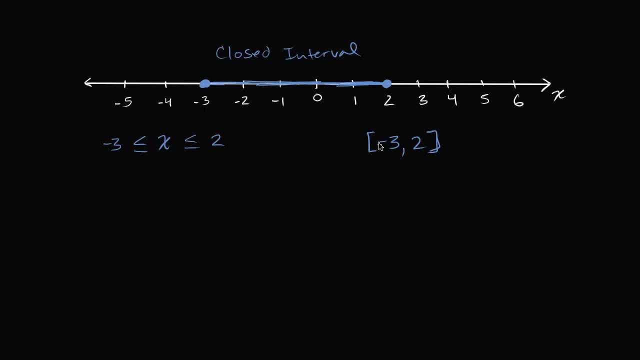 that we include. so this bracket on the left say that we include negative three and this bracket on the right says that we include positive two in our interval. Now, sometimes you might see things written a little bit more mathy. You might see something like that, like: 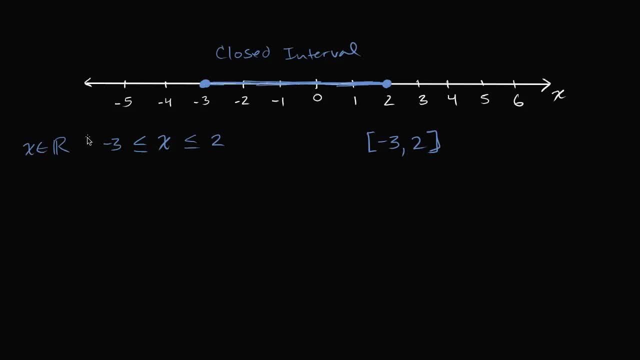 x is a member of the real numbers, such that. So- and I could put these curly brackets around like this: These curly brackets say that we're talking about a set of values and we're saying the set of all x's that are a member of the real numbers. so this is just fancy math notation. 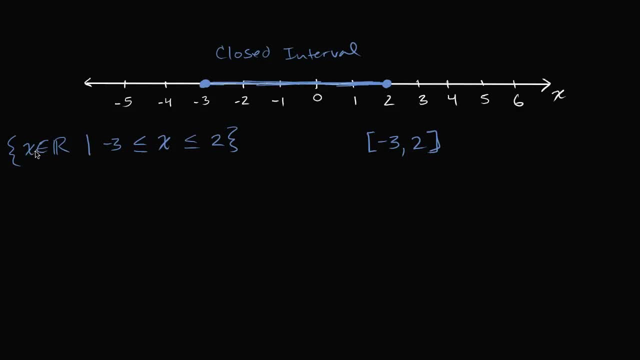 it's a member of the real numbers- I'm using the Greek letter epsilon right over here. It's a member of the real numbers such that this little, this vertical line here, means such that negative three is less than x is less than. 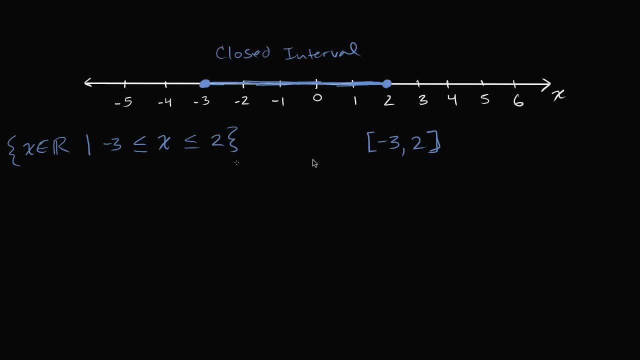 negative. three is less than or equal to. x is less than or equal to two. I could also write it this way: I could write: x is a member of the, the real numbers, such that x is a member, such that x is a member of this closed set. I'm including: 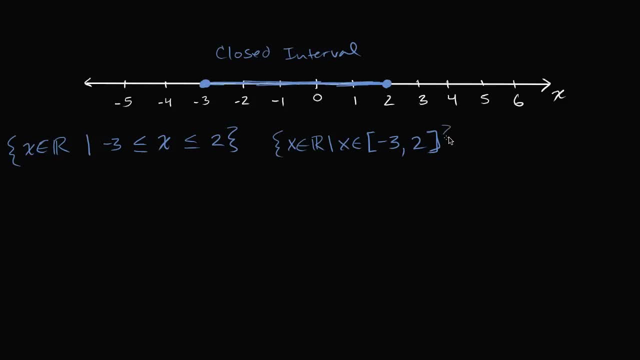 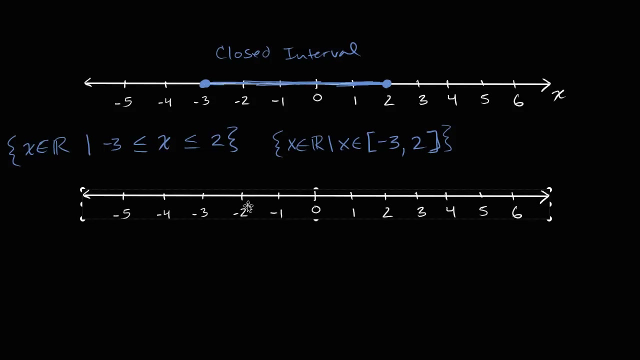 I'm including the end points here. So these are all different ways of of denoting or depicting the same interval. Let's do some more examples here. So let's let me draw a number line again. So number line, and now let me do, let me just do- an open interval. 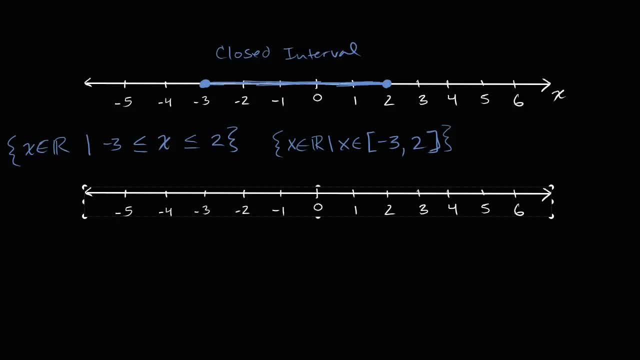 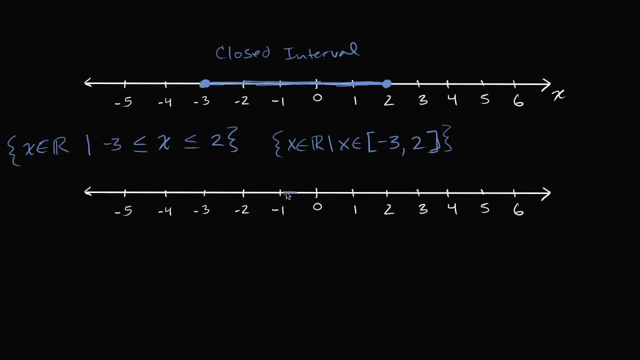 an open interval just so that we see. we clearly can see the difference. So let's say that I want to talk about the values between negative one and four. negative- let me do this in a different color- So the values between negative one and four. 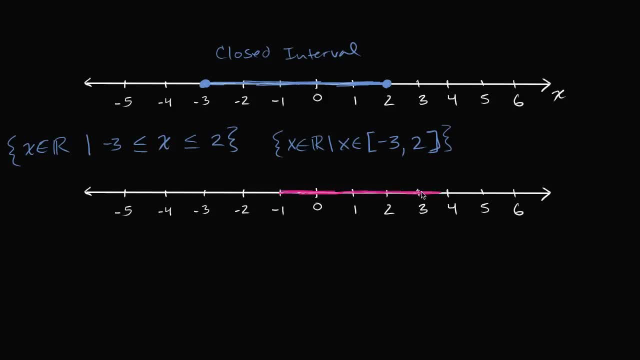 but I don't want to include negative one and four. So this is going to be an open interval. So I'm not going to include four and I'm not going to include and I'm not going to include negative one. Notice, I have open circles here. Over here I had closed circles, The closed. 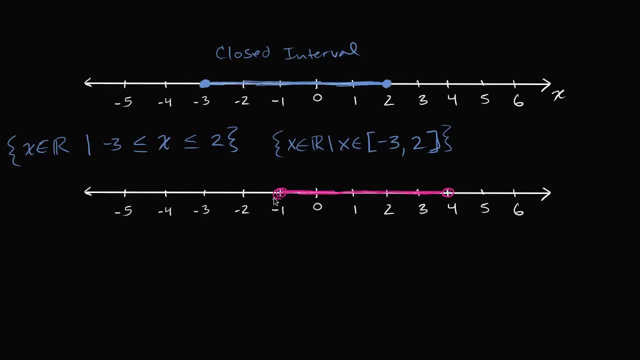 circles told me that I included negative three and two. Now I have open circles here, So that says that I'm not. it's all the values in between negative one and four, So negative one or negative point nine, nine, nine, nine, nine, nine, nine is going to be. 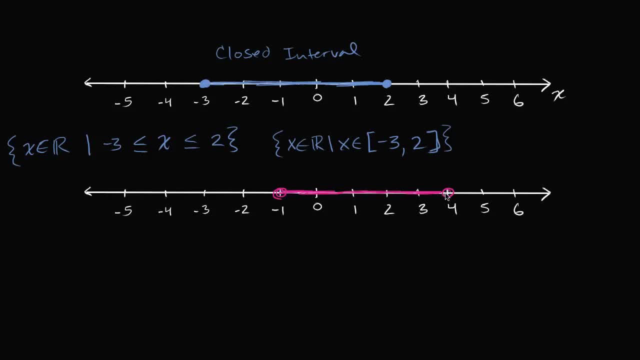 included, but negative one is not going to be included. And three point nine, nine, nine, nine, nine, nine, nine is going to be included, but four is not going to be included. So how would we what? what would be the notation for this? Well, here we could say: 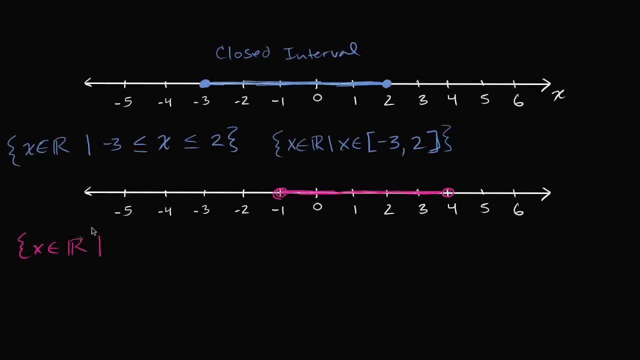 x is going to be a member of the real numbers, such that negative one. I'm not going to say less than or equal to, because x isn't, x can't be equal to negative one. So negative one is strictly less than x is strictly less than four. 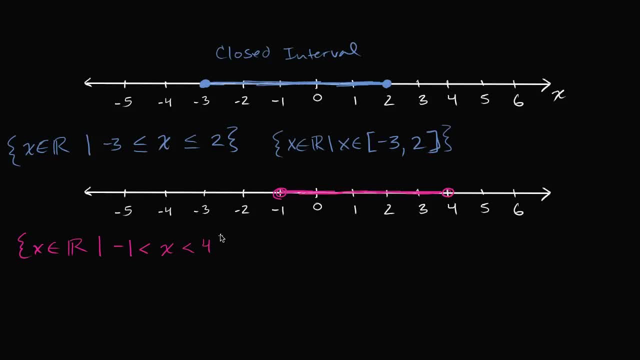 Notice not less than or equal, because I can't be equal to four. Four is not included, So that's one way to say it Or another way. I could write it like this: X is a member of the real numbers, such that x is a member of now, the 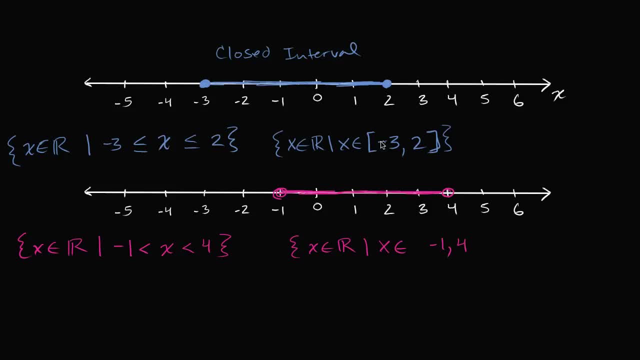 interval is from negative one to four. but I'm not going to use these brackets. These brackets say, hey, let me include the endpoints, but I'm not going to include them, So I'm going to put the parentheses right over here. Parentheses. So this tells us that we're dealing with an open. 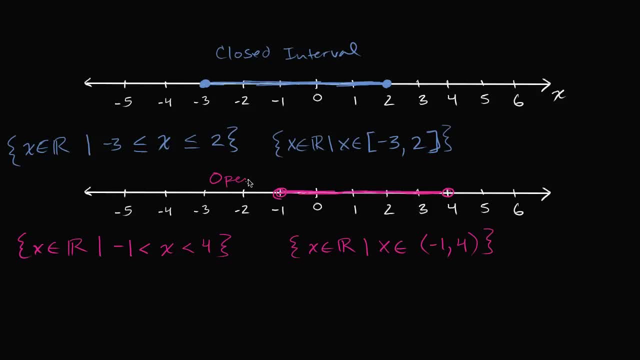 interval. So this right over here. let me make it clear: this is an open, an open interval. Now you're probably wondering: okay, in this. in this case, both endpoints were included. it's a closed interval. In this case, both endpoints were excluded. it's an open interval. 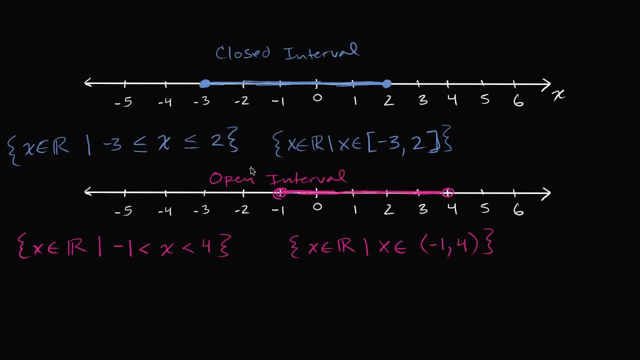 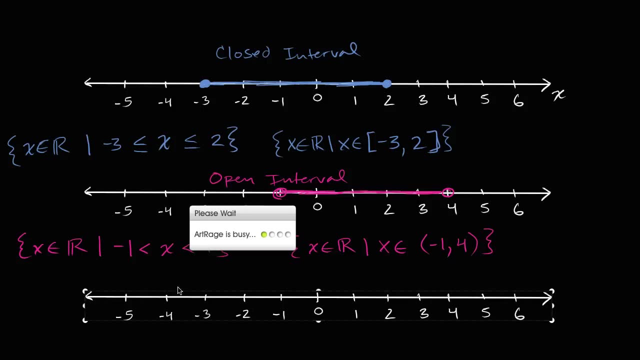 Can you have things that have one endpoint included and one endpoint excluded? And the answer is absolutely. Let's see an example of that. So I'll get another number line here, Another, another number line, And let's say that we want to. 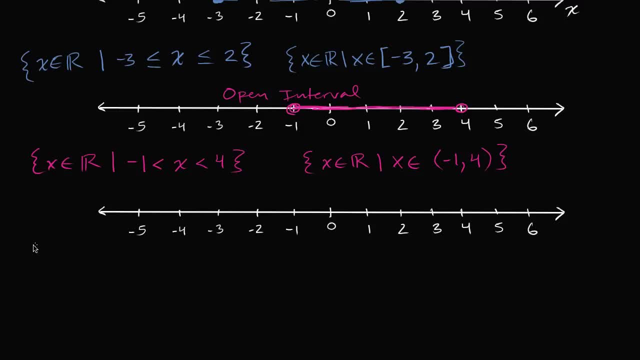 actually, let me do it the other way around. Let me write it first and then I'll graph it. So let's say we're thinking about all of the x's that are a member of the real numbers, such that, let's say negative four, let's say negative four is not included, is less than x. 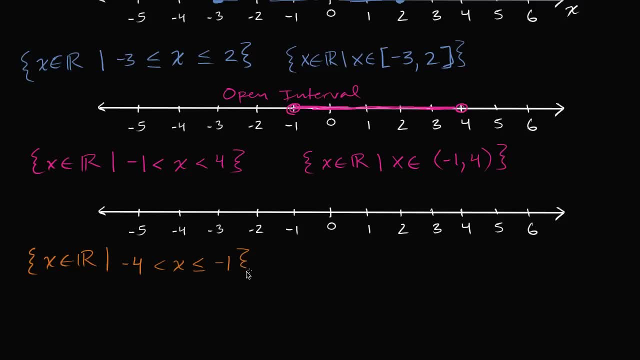 is less than or equal to negative one. So now negative one is included. So we're not going to include negative four. Negative four is strictly less than, not less than or equal to. So x can't be equal to negative four, so open circle there. But x could be equal to negative one. it has to be. 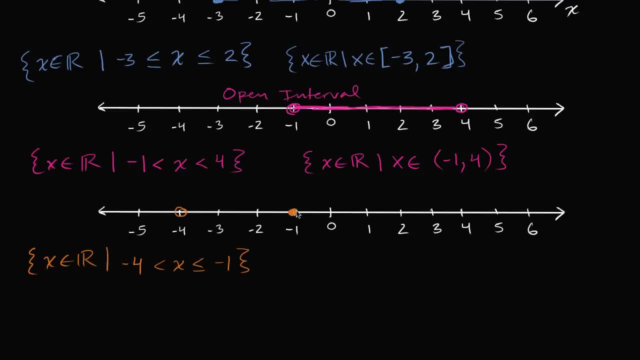 less than or equal to negative one, So it could be equal to negative one. so I'm going to fill that in right over there And then it's everything in between. If I want to write it, this notation I could write: x is a member. 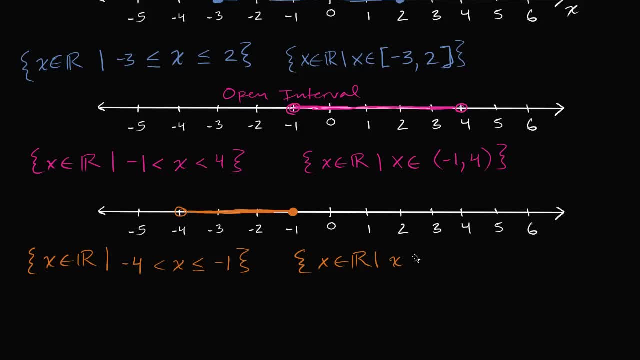 of the real numbers, such that x is a member of the interval. So it's going to go between negative four and negative one, But we're not including negative four. We have an open circle here, so I'm going to put a parenthesis on that side. 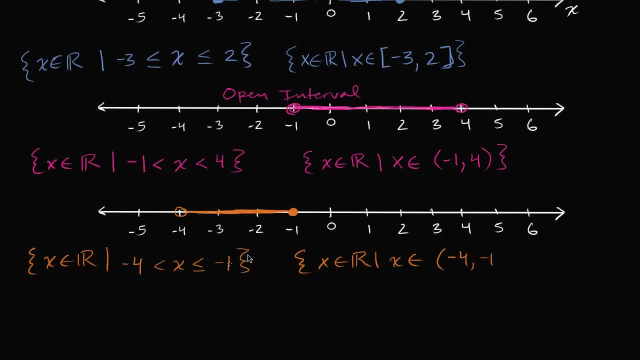 But we are including, we are including negative one, We are including negative one, So we put a bracket on that side, And so that would be that. right over there would be the notation. Now there's other things that you could do with interval notation. You could say: well, hey, everything. 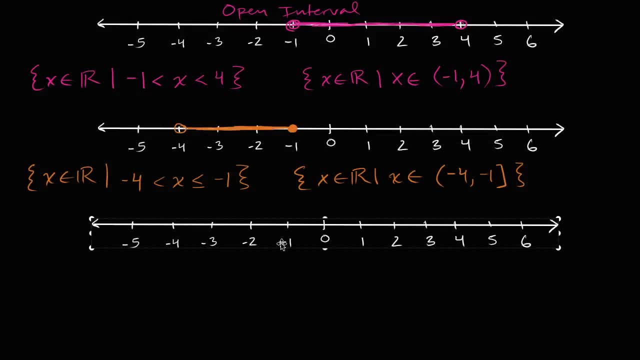 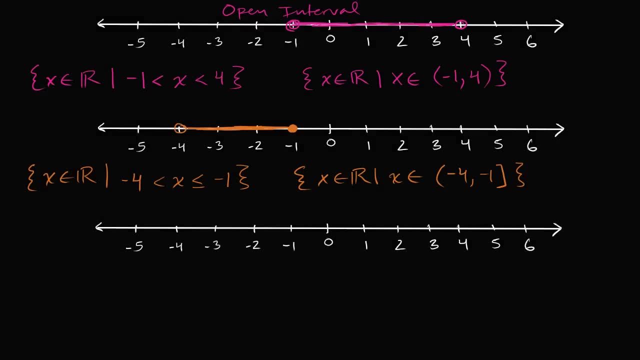 except for some value. So let me give another example. Let's get another example here. Let's say that we want to talk about all the real numbers except for one. So we want to include, so we want to include all of the real numbers, all of the real numbers. 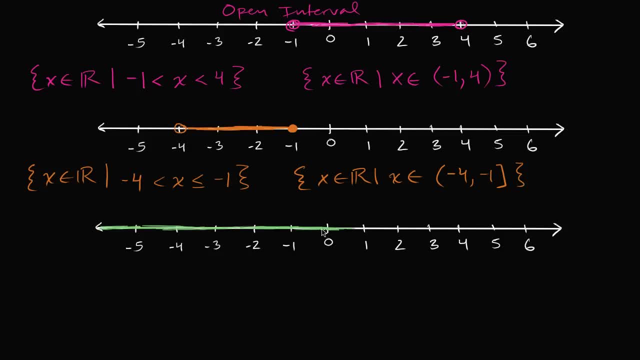 except, except for one, Except for one. So we're going to exclude one right over here. So open circle. But it could be any other, any other real number. So how would we? how would we, how would we denote this? 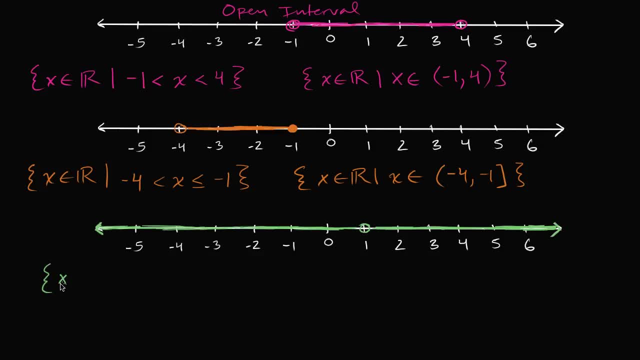 Well, we could write. we could write: x is a member of the real numbers, such that x does not equal, does not equal one. So here I'm saying, look, x can be a member of the real numbers, but x cannot be equal to one. It can be anything. 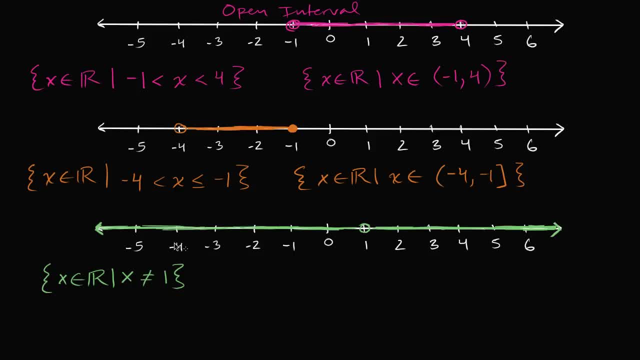 else, but it cannot be equal to one And there's other ways of denoting this exact same interval. You could say, you could say x is a member of the real numbers, such that x is. you could say such that x is less than one, or x is: 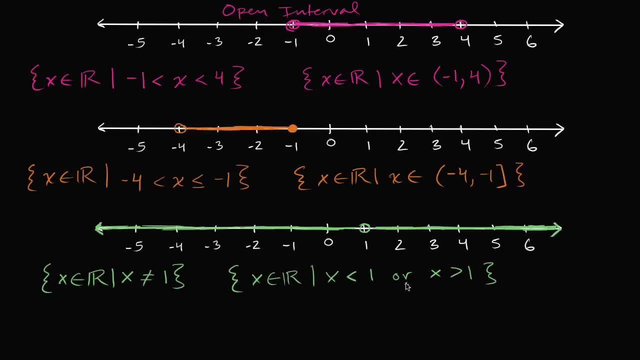 greater than one. So you could- you could write it just like that, Or you could do something interesting. This is probably this is the one that I would use. This is the shortest and it makes it very clear. Say, hey, everything except for one. But you could even do something. 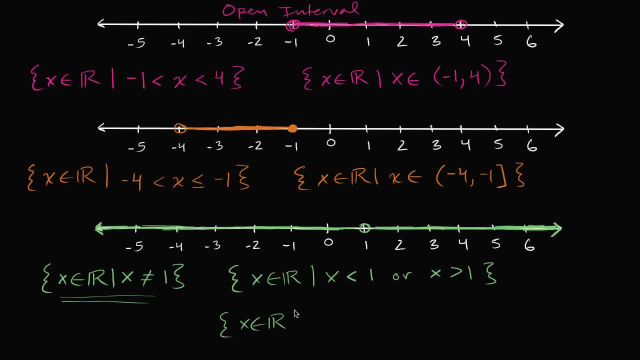 fancy. like you could say, x is a member of the real numbers, such that x is a member of the set going from negative infinity to one, not including one. Or x is a member of the set going from, or a member of the interval going from one not including. 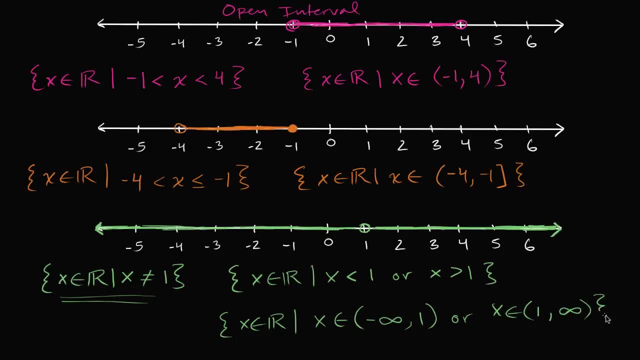 one all the way to positive, All the way to positive infinity. And when you're talking about negative infinity or positive infinity, you always put a parenthesis And the view there is: you can never include everything all the way up to infinity. It's. 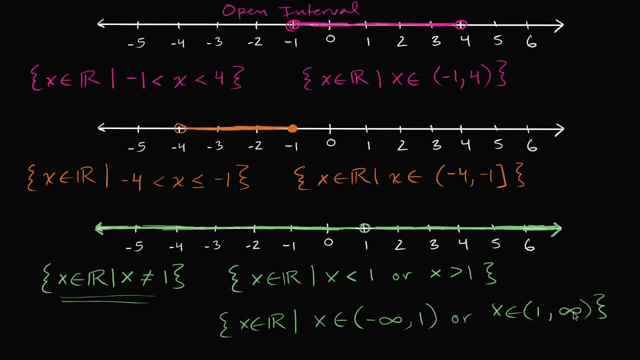 needs to be at least open at that end point, because infinity just keeps going on and on. So you always want to put a parenthesis if you're talking about infinity or negative infinity. It's not really an end point. It keeps going on and on from there.